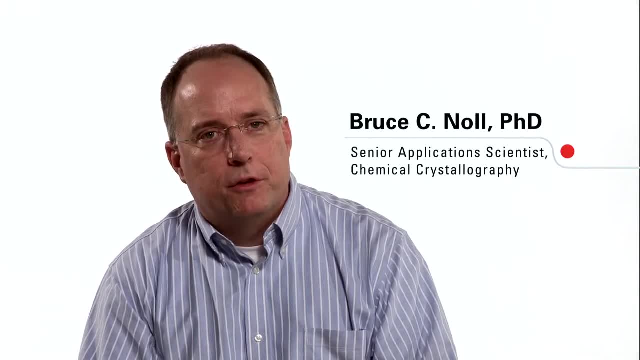 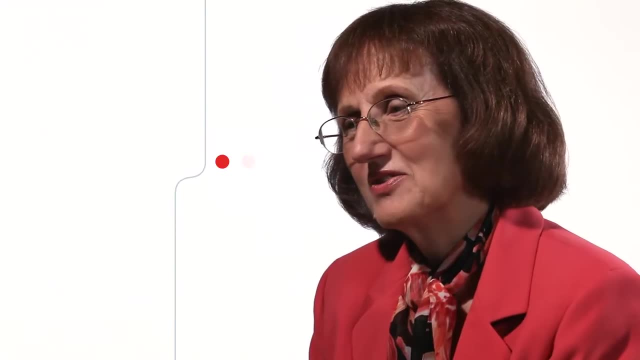 else in the world the shape of a molecule, to see what a molecule truly is. The crystallographer really is the first person to ever know exactly what this thing looks like As far as the highlights in the development of chemical crystallography over the history. 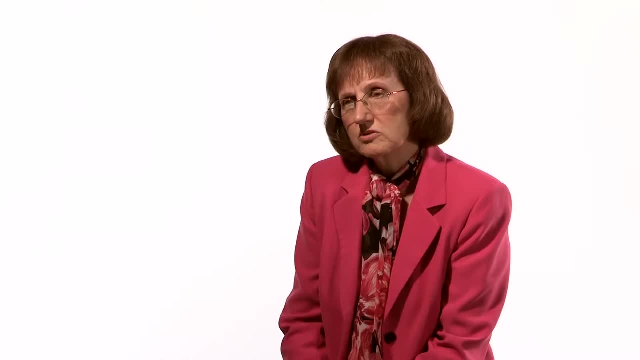 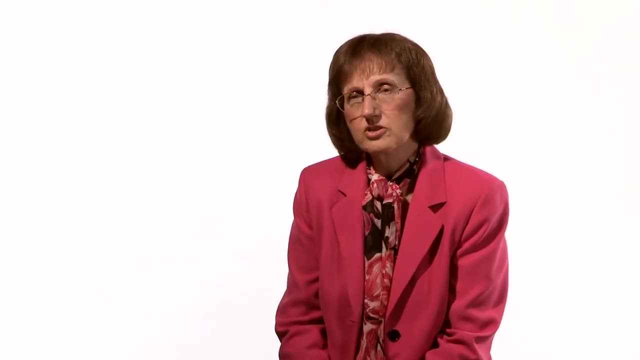 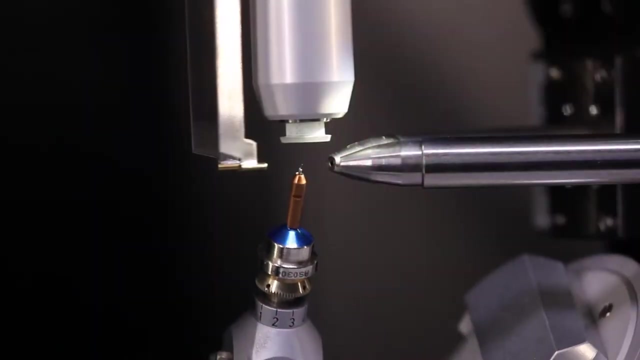 of our company, I think as well- development of two-dimensional detector technology. always we've pioneered that. The multi-wire detectors were a revolution in protein crystallography in the 80s and the two-dimensional CCD was a revolution in chemical crystallography. 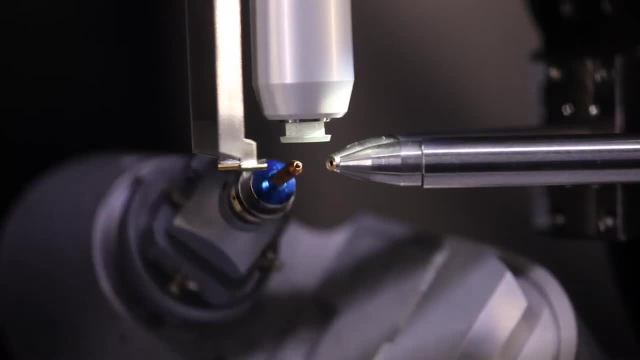 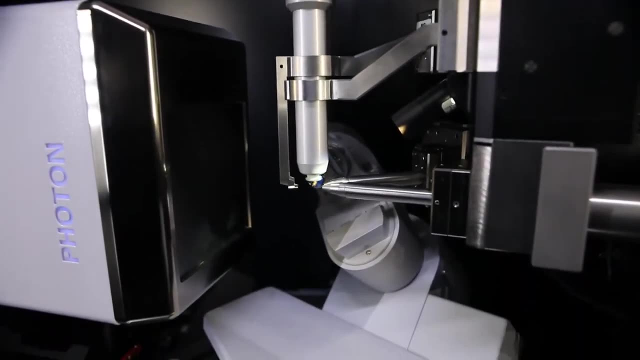 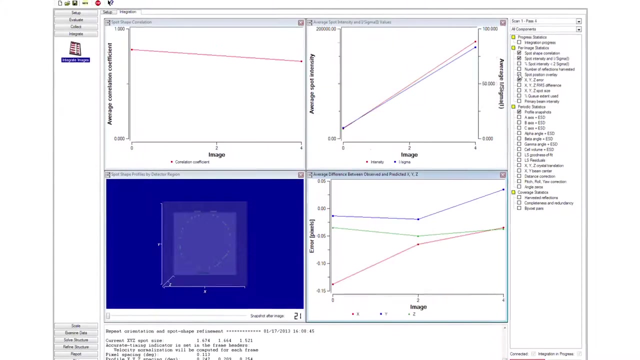 in the 90s We did not even perceive How good those detectors were going to be. And now we're in the midst of another revolution with the CMOS on the two-dimensional detectors. And all of these are embedded together with really fantastic software. The software is what makes all this interesting hardware work. 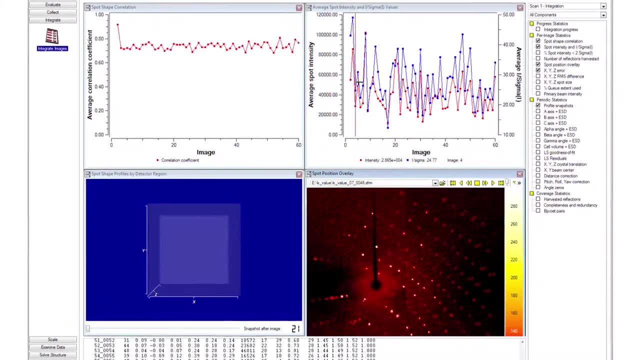 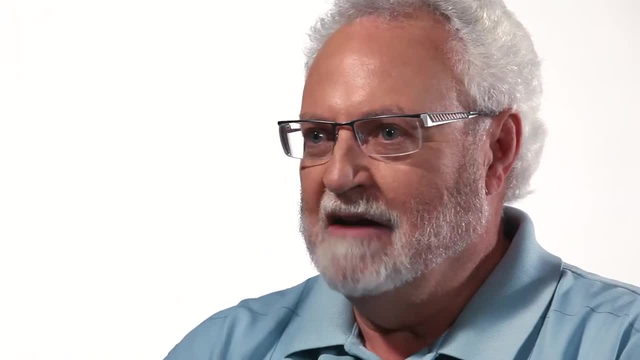 although it's sometimes buried deep in the systems and people may not perceive how critical the role of the software is. What's important if you're a customer is you first of all have to be able to solve your problems, and that means you have to collect extremely good data, but you also have to 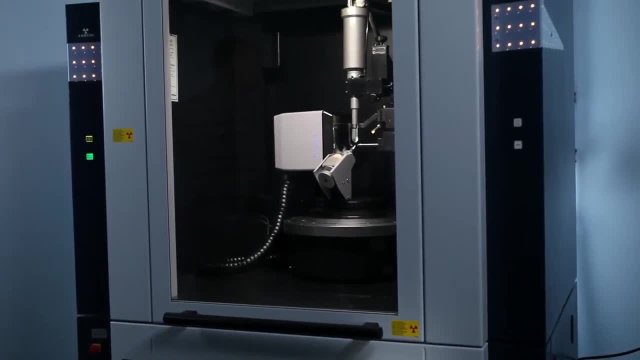 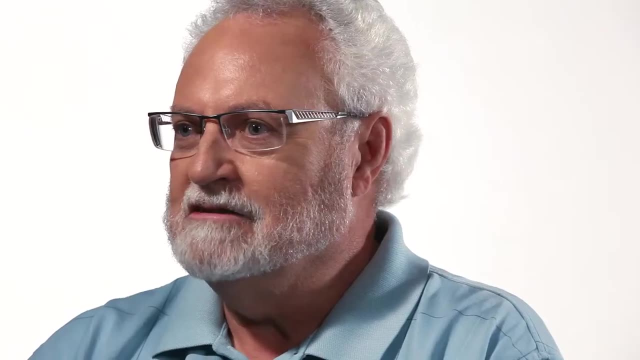 have an instrument that's very reliable, it doesn't have service issues, you don't have to change components by hand and these things, and it also has to be pretty straightforward to operate and it has to give you publication quality data with a minimum of effort. 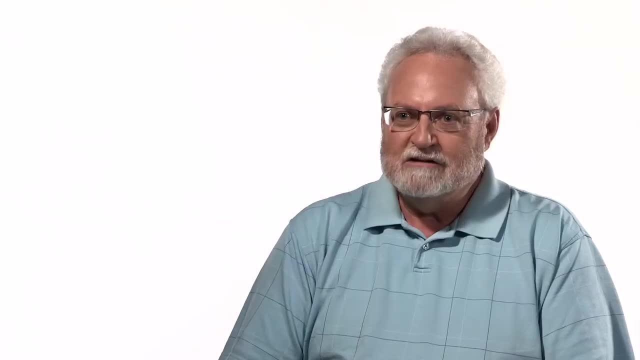 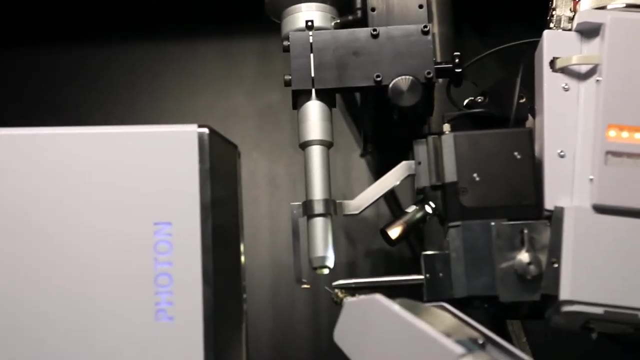 So our newest generation of instruments from Bruker has tried to address all of these with a modular design of all of the components, a state-of-the-art new detector technology and automated software which could be used for any kind of problem, ranging from simple. 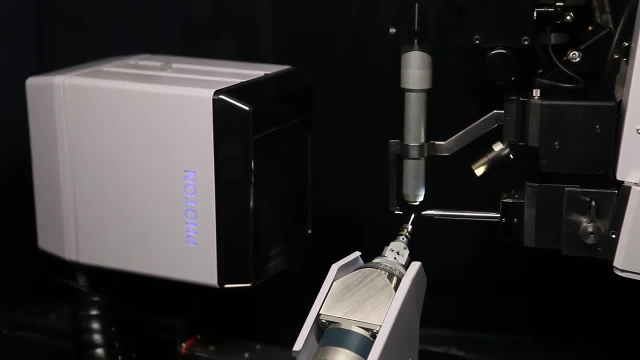 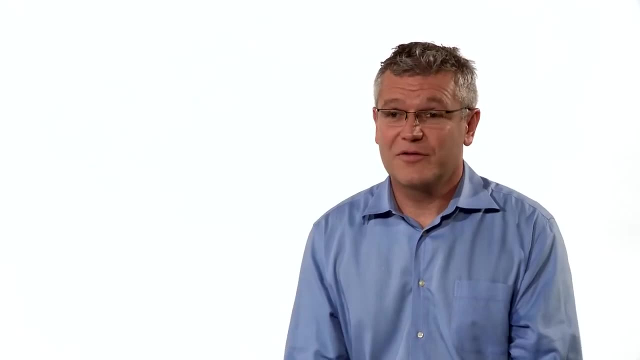 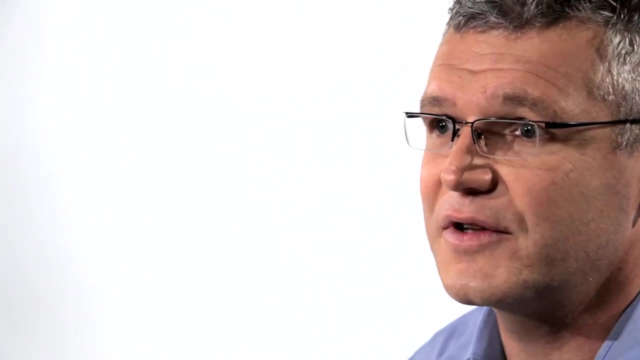 structures for undergraduate students to very complicated research problems in any of our laboratories around the world. Bruker has really a great track record of being the technology leader. Bruker is considered to be the detector company and when you look at detectors that have come out of this company,